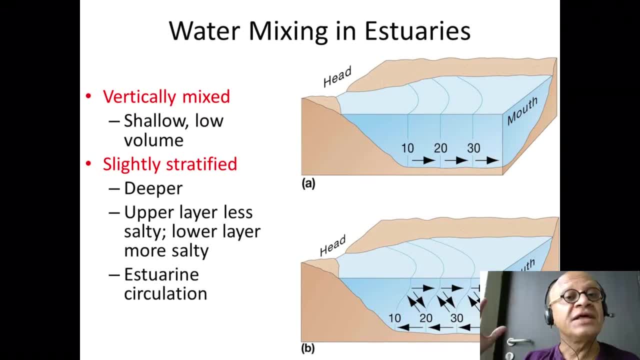 So we said, estuaries are basically semi-enclosed, so they have ocean water coming in and fresh water coming in right. They could also be evaporative estuaries, of course, but nonetheless this means there is a mixing issue involved. 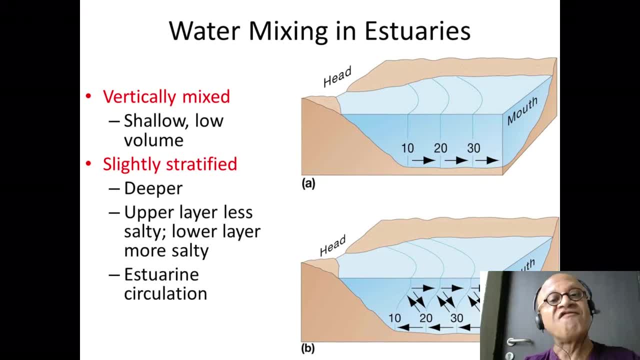 This obviously depends broadly on the volume of water coming in and the depth of the estuary, which create the relative densities of the surface waters and the deeper waters. So the normal estuarine flows tend to be that heavier marine water. ocean water flows in at the bottom. 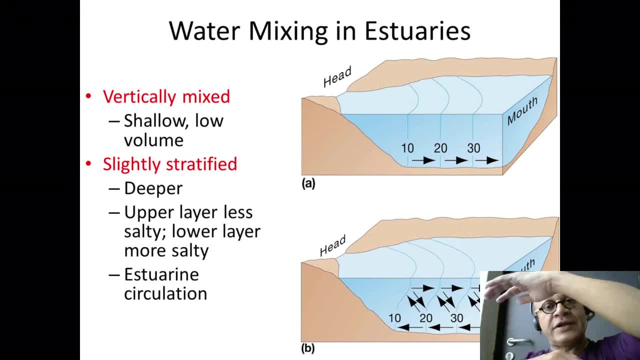 The fresher water coming from land tends to flow out at the top. We'll see that there are exceptions to this, But nonetheless, When the estuary is fairly shallow and the fresh water flow is not that high, the winds are able to mix it up and the density contrast is not so strong. 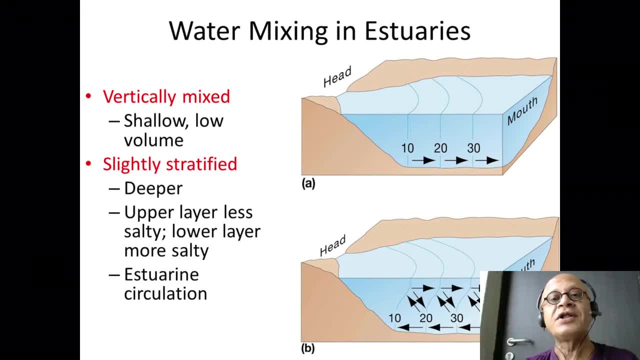 So you end up with this kind of a vertically mixed estuary. So you can see that the salinity is fairly well mixed down to the bottom, which is shallow, 10,, 20 parts per thousand, 30 parts per thousand- to the mouth of the estuary where it mixes with the ocean. 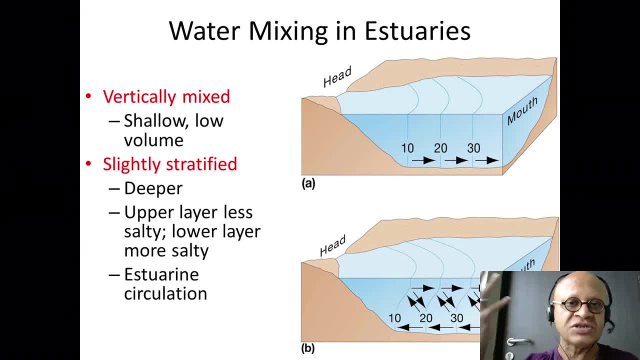 And becomes the normal ocean water, which is usually around 34, 35 parts per thousand, as we learned before, correct. So if you have a deeper estuary then you can have a slightly stratified. So you can see here fresh water is flowing out farther near the surface, whereas the ocean water with higher salinity is coming in at the bottom. 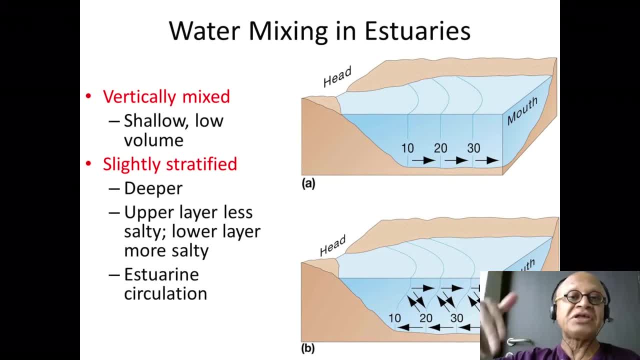 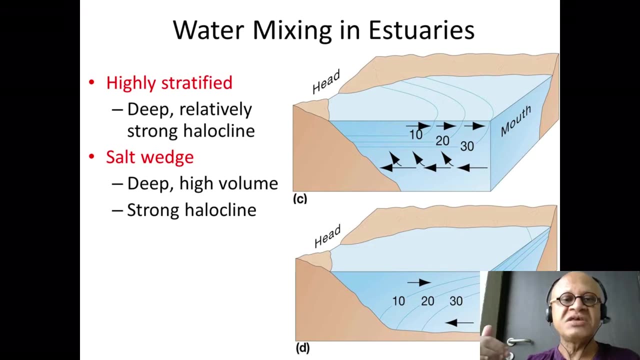 And there is Cross-mixing happening in the vertical direction. depending on how much mixing there is, how much evaporation happens and what is the volume of the flow, and so on. Broad categories- just remember the terminologies. Highly stratified- when the estuary is deep and you have a relatively strong halo-cline, then the ocean water doesn't mix so much with the surface. 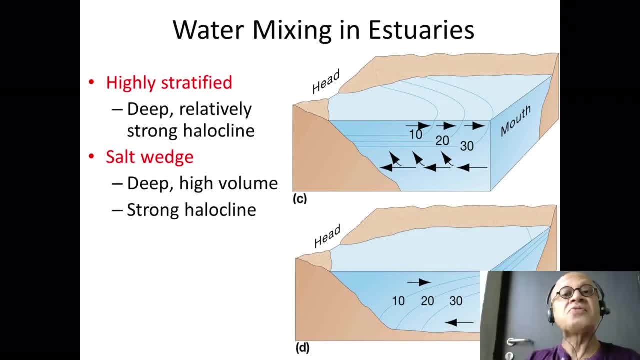 This again depends on what is called surface turbulent kinetic energy, which is a combination, The combination of cube, of the wind speed, because wind can stir the water- and buoyancy. forcing means heating or cooling, For example. heating will make the surface warmer and stratify the water more. 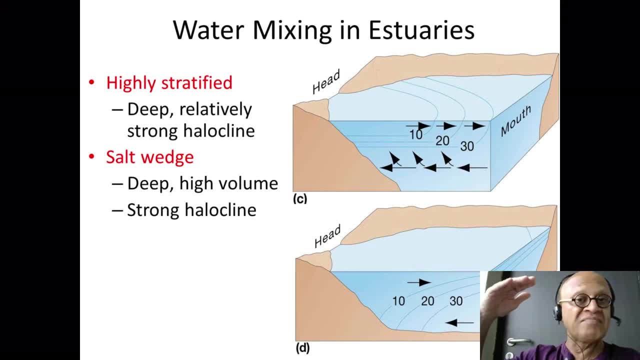 Whereas cooling, let's say by evaporation or winter time heat loss, can make the densities heavier and can facilitate mixing. So highly stratified here Shown salinity decreasing again towards the mouth And heavier water coming in and very little vertical mixing. 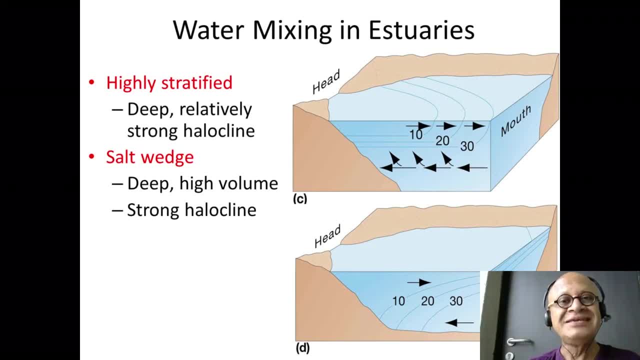 You get a salt wedge when a very deep, very high volume of water comes in to the head of the estuary and basically pushes against the ocean water and creates this heavy salt wedge. You can see here the brackish water of 10 parts per thousand is going all the way to the mouth of the estuary. 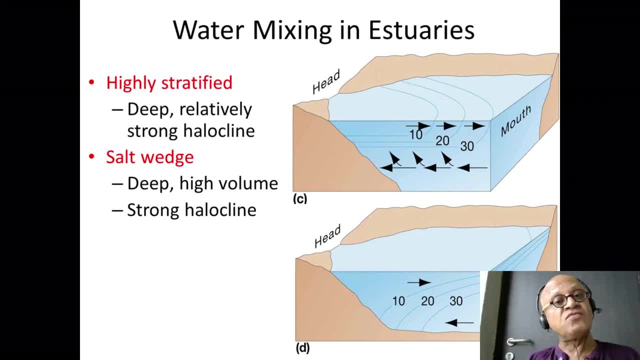 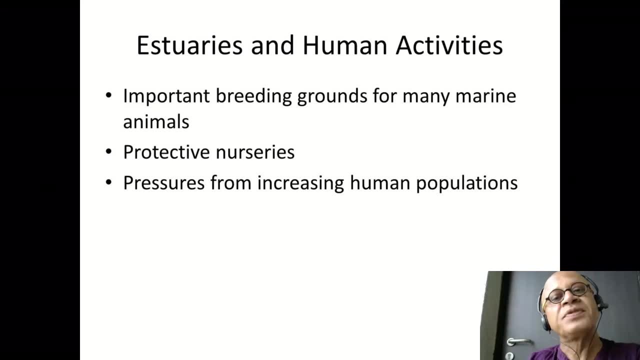 Okay, And the ocean water is being restricted closely. It's being restricted close to the mouth of the estuary and it's mixing up with this high volume of fresh water. Okay, So quickly moving on to the estuaries and human activities. 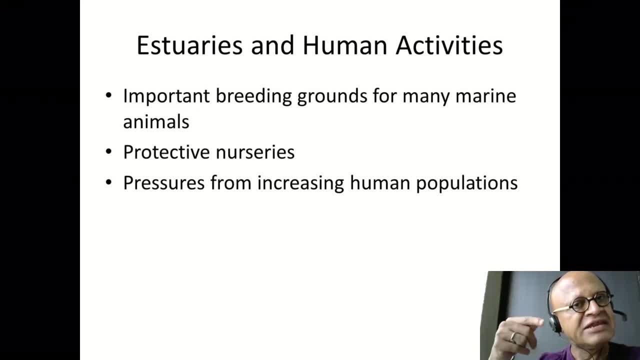 I mentioned a couple of things: The salinity and its effects on the coastal waters, Runoff and snow melt, for example. So even in a monsoon region like the Bay of Bengal, rain happens during the summer And the river runoff peaks. 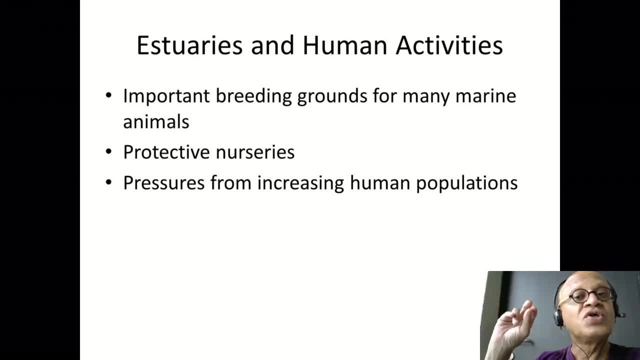 A little bit after that. So the species that live in the estuaries or open ocean and come to the estuaries for some part of their life cycle Are used to these seasonal variability in level of salinity, Which is also often related to the level of oxygen in the water. 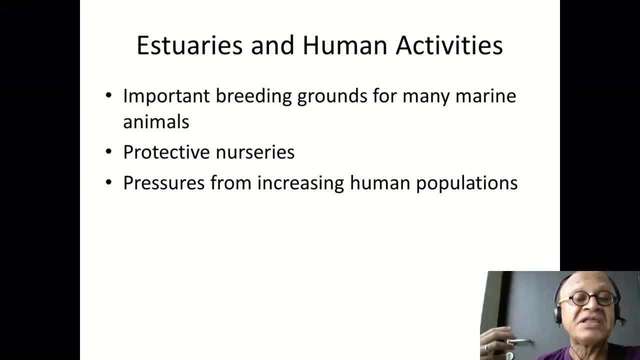 Because the oxygen is also dependent on how much sediment there is, How much mixing happens, etc. etc. Right Mixing is like ventilation, So the oxygen in the atmosphere, which is high, gets mixed into the water when there is mixing, So you can have highly stratified water. 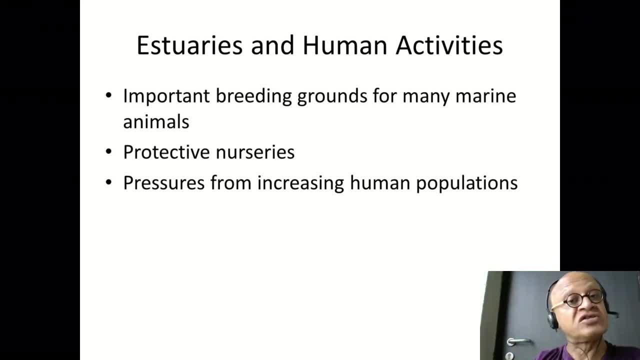 Then the bottom waters can get very low in oxygen, as we will see a little bit later on. That is not good for life. So important breeding grounds for many marine animals does occur in the estuaries. Crabs, things like that, live on the bottom. 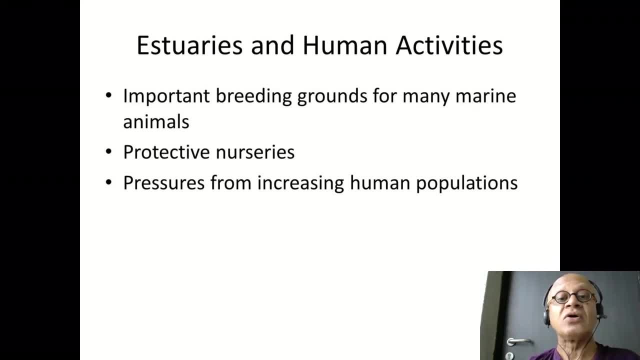 Or they are reef builders, like oysters, Clams and so on. They cannot move very fast, So if you start to perturb the system, then you begin to kill them. Okay, Whereas some fish can of course run away, But their life cycle can get disrupted if there are perturbations by human activities. 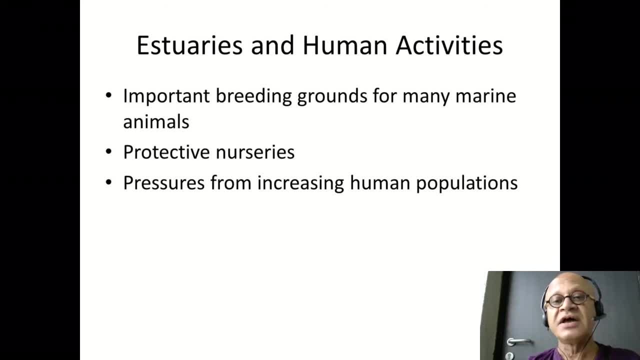 So there are many protective nurseries And the human populations moving closer and closer to the coast And increasing agriculture on land, Deforesting, urbanizing etc. Obviously putting a lot of pressure on these valuable nurseries, biodiversity and so on. 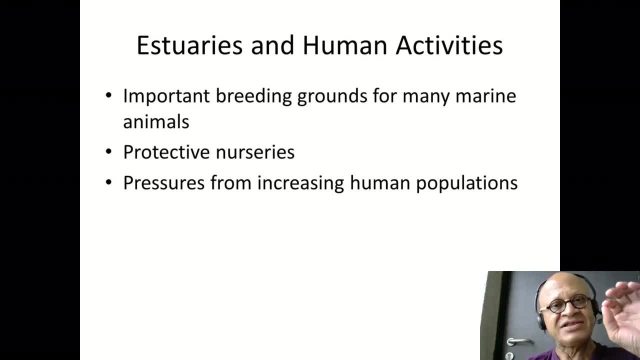 Okay And those are very finely balanced, Because when a fish, let's say, goes and lays eggs, It wants to make sure that the eggs just don't float away. They have to be, circulation has to be such that they have to be contained. 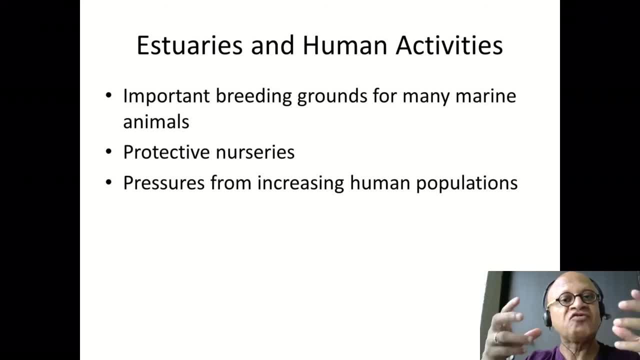 And the salinity conditions, friction etc have to be certain levels, Like the grunion we saw, which were hatching the eggs during the spring tide in the sand, for example, Right. Those are very finely tuned evolutionary features And when the eggs hatch, the larvae immediately start looking for food. 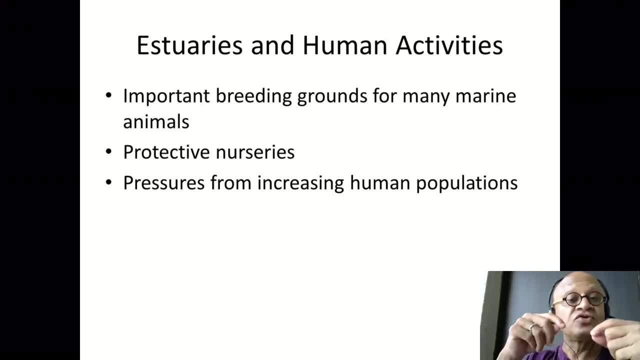 But there are other creatures which want to eat the larvae. So the evolution has optimized all these things: Circulation, Food evolution, Availability, Predation, pressure And so on. So when humans perturb the system, they perturb all these things. 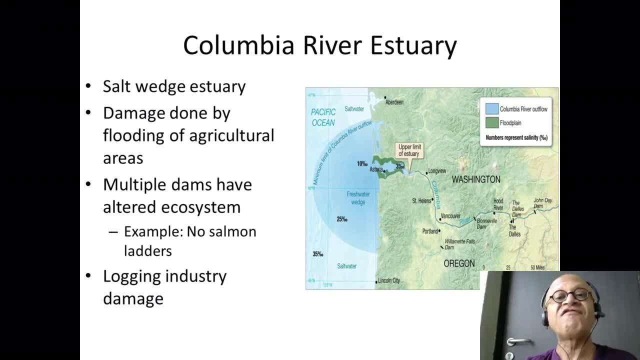 Okay, So Columbia River estuary is one fine example. There are others that we will look at: Ganga, Brahmaputra, Nile, Mississippi and so on. So it produces this big salt wedge estuary by bringing in so much water. 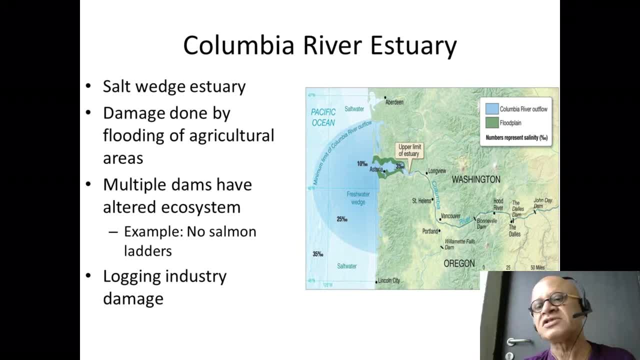 Of course, there have been tons of dams built. You can see there are many, many, many dams built And that reduces the sediment flow as well as the water transport coming into the ocean at the end. So damage also done by the agricultural land here.